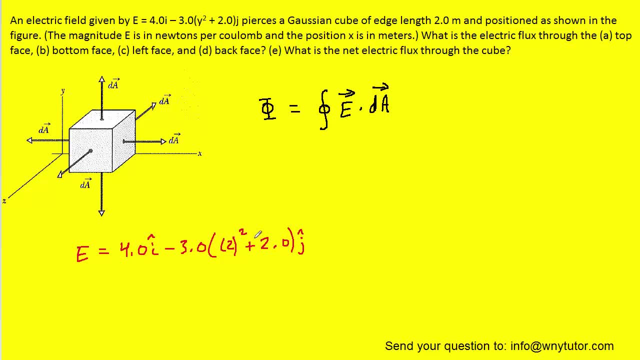 two. We can simplify inside the parentheses because we have four plus two, which is six, and then multiply that by the three, So we'll actually have a minus 18 j-hat for the j-hat component and then the 4.0 i-hat. So once we have the electric field, that is. 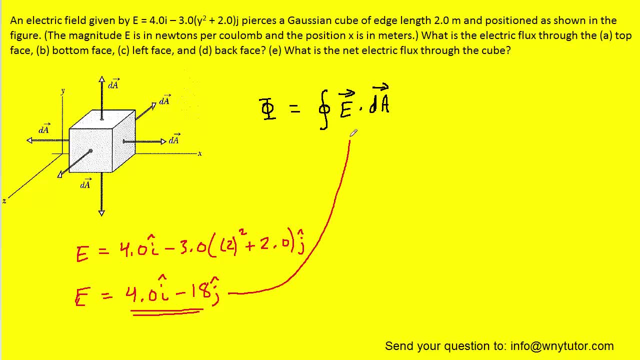 flowing through the top surface of the cube. we can plug that in to our integral. And now we want to make a note about this differential area vector right here. Since we're calculating the electric flux through the top surface of the cube, this dA term is simply going to equal 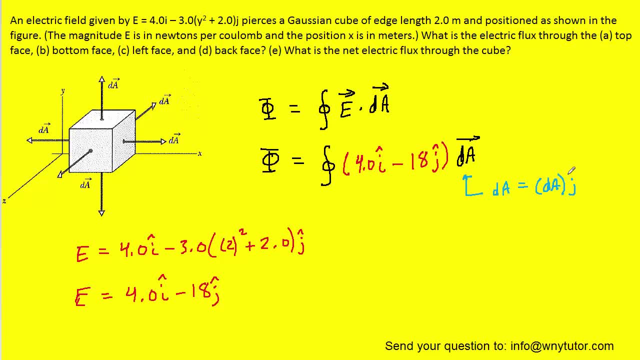 dA for the j-hat component. Now we can say that again, because we're only interested in calculating the electric flux through this top surface And we can see that the dA vector is pointing in the positive y direction, which of course is represented by the j-hat notation. So we're going to substitute 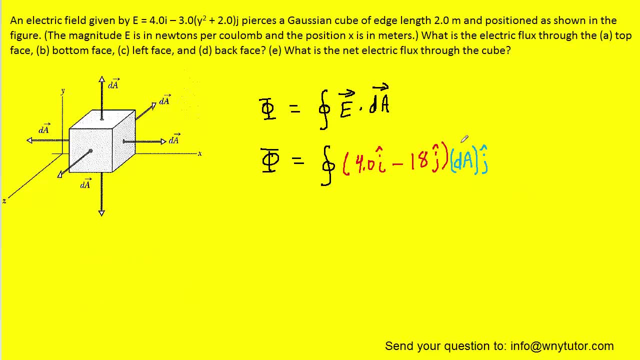 this dA with this expression dA j-hat. Next, we will distribute into the parentheses on the left-hand side, and what we want to note- and this is the result of the rules of taking dot products- is that when we multiply a j hat by an i hat component, they effectively cancel each other out. so you're really 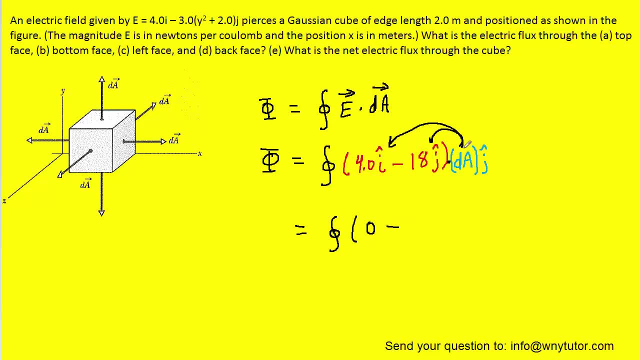 left with just zero here, and then also, according to the rules of taking dot products, when we multiply j hat components, those effectively cancel. so what we have is a minus 18, and then da here, and of course this is negative 18 inside the parentheses. and since negative 18 is a constant, 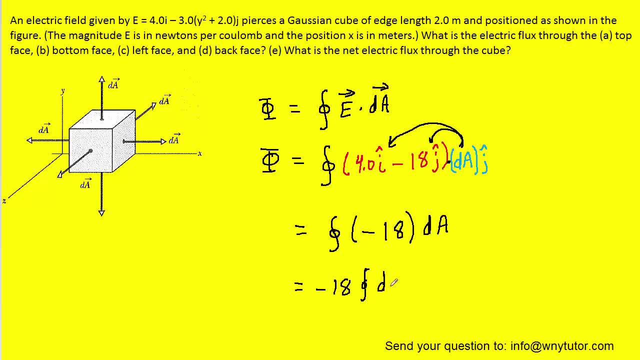 we can remove it to the outside of the integral and then we're left to integrate this da. now, of course, the integral of da is just the area itself, so we have negative 18 multiplied by the area. now the area of the top face, because it's a square, is just going to be 2 times 2, so we can substitute. 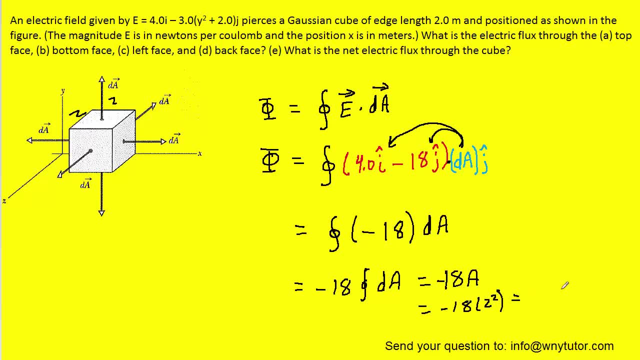 that in for the area. we can write that as 2 squared and then when we simplify that, we get negative 72 and the unit. if we go back to the original definition of flux, it's an electric field multiplied by the area of the top face, and then we can substitute that in for the area of. 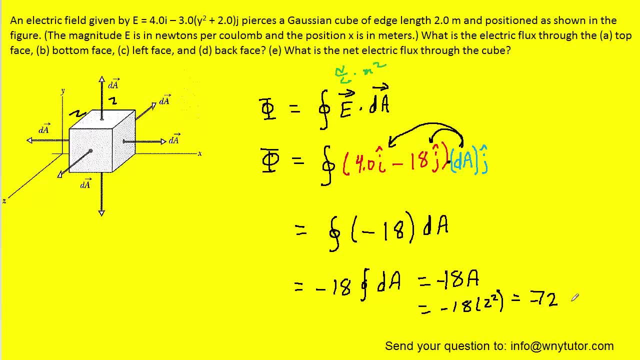 the bottom face, and then we can substitute that in for the area of the top face and then we can multiply that by the area. now, of course, electric field is newtons per coulomb and area is meters squared. so we're going to have negative 72 newton meters squared per coulomb. this would be the final. 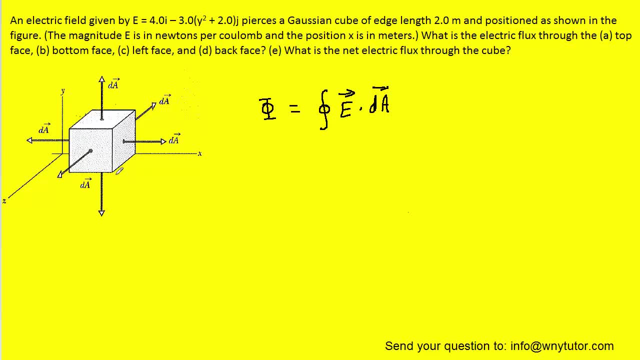 answer to part a, we now go on to part b, which wants us- wants us- to calculate the electric flux through the bottom face. it's a little bit obscured, but here we have the bottom face, which is once again a square. now we'll notice that the y coordinate of that bottom face is actually zero. 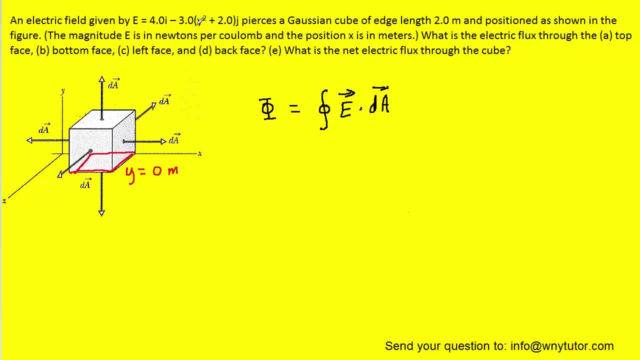 meters, and so we'll plug zero in for the y in our electric field and then we'll have a square equation. and then we'll simplify: inside the parentheses we would just have two, and then we multiply it by the minus three, so our electric field becomes 4.0. i hat minus 6.0. j hat that's. 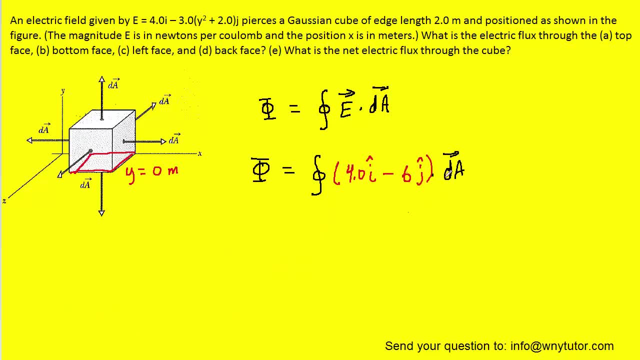 the expression for the electric field that will plug in to our integral, and then for the da, because we're calculating the flux to the bottom surface, we note that the da is projecting downward in the y direction. so we're going to have negative 72 and then we're going to have negative 72, and then 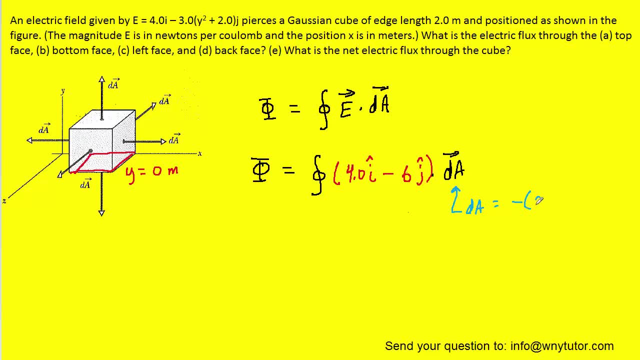 we know that this da can be substituted with negative da j hat. of course it's negative because it's pointing in the y direction, downward. as before, we'll have to distribute and, as before, an i hat multiplied by a j hat is zero, and then a j hat times a j hat. those j hats just cancel out. 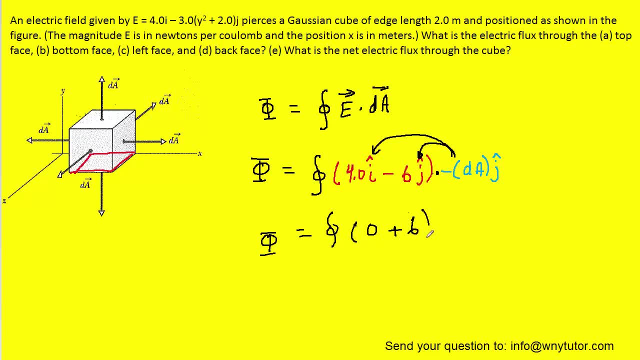 so we're also multiplying a negative by a negative. so this is actually plus 6 and then we have da. that can simplify to just the integral of 6. da we'll pull the 6 out and then the integral of da is just going to equal the area and, just like before, the area of the bottom face is: 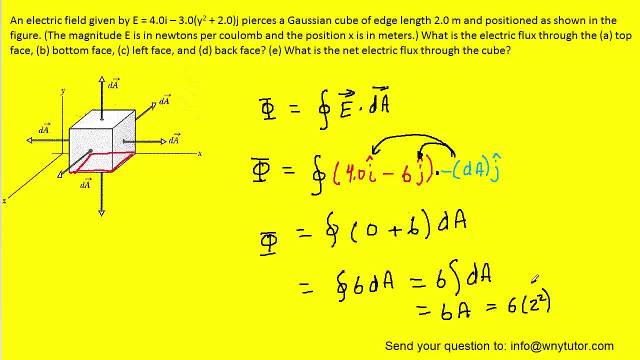 going to be 2 by 2 or 2 squared, and so when we finish this one off, we're going to have 24 newton meters squared per coulomb. so this would be the correct answer to part b. we'll proceed in a similar way for the left face. notice that the left face, because it extends. 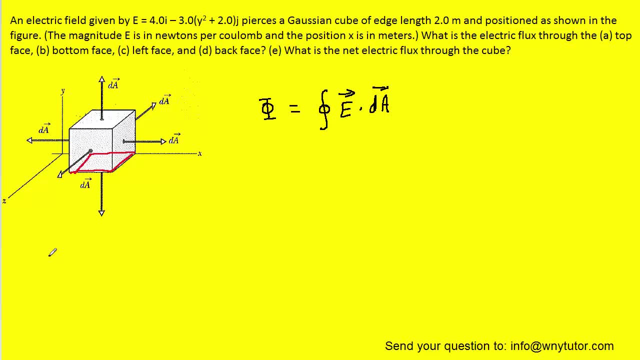 vertically has a variable y component, and so we can't, like we did before, set a particular value for y, because it kind of varies from 0 all the way up to 2, but, as we'll see, that will actually not matter because it's going to cancel away. so let's set up the electric. 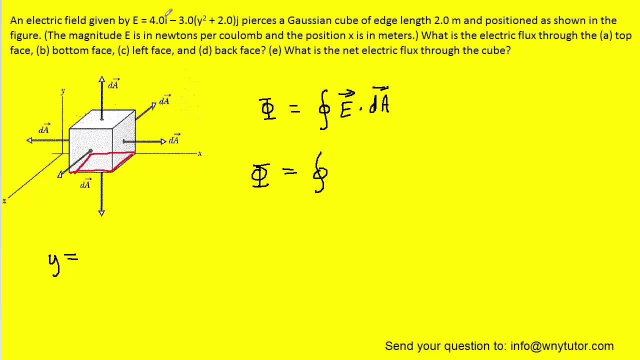 flux and this case for the electric field. we'll just use this entire equation here now, because we're determining the electric flux through the left face of the cube. we can say that da- hopefully able to squeeze it in here- is going to be da multiplied by negative. i hat notice it's. 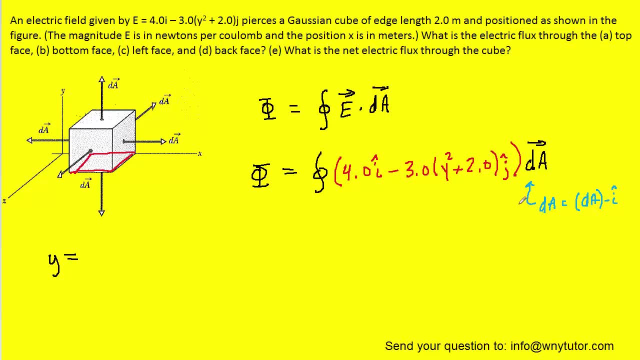 negative because the da vector is pointing to the left and it's i hat because it's pointing along the x direction. so we'll make that substitution. so now we'll have to distribute again and when we multiply the negative i hat and the i hat, the i hats are going to cancel, so we'll write the. 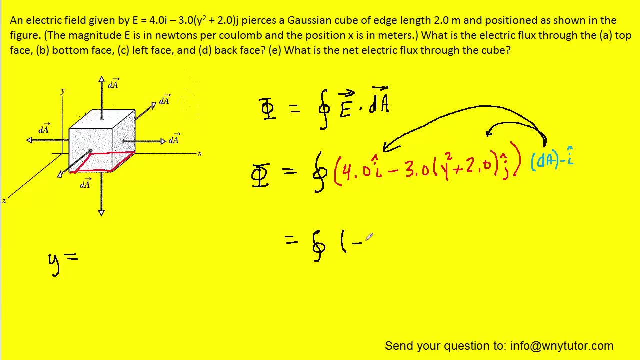 integral as follows: we'll have a negative 4.0. notice: it is negative because we're multiplying a negative by a positive and then, conveniently, the i hat multiplied by j hat cancels away. so this is actually just minus zero, which we don't even have to write. we can just leave it as negative. 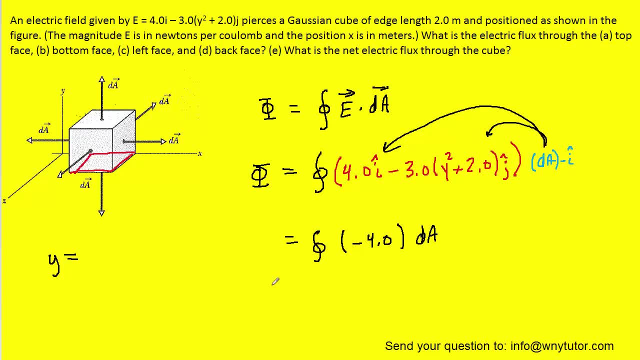 4.0 and then we have the da. the rest is the same. we can pull out the negative 4.0 and then integrate. so we're going to have negative 4.0 multiplied by the area. the area once again is just 2.0 squared. 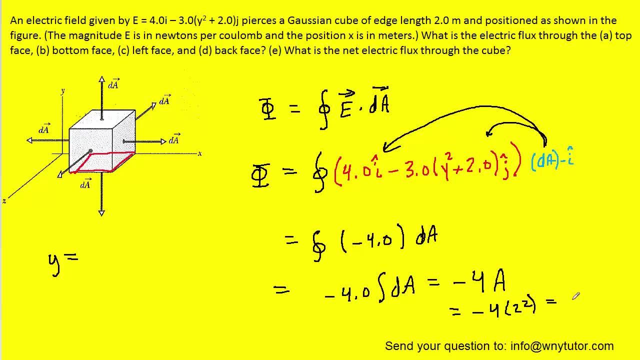 and so we're going to be left with negative 16.0 and then the unit of newton meters squared per coulomb. so this would be the correct answer to part c of the question. on to part d- and there's a bit of a shortcut for this one- they're asking for the flux along the back face of the cube. 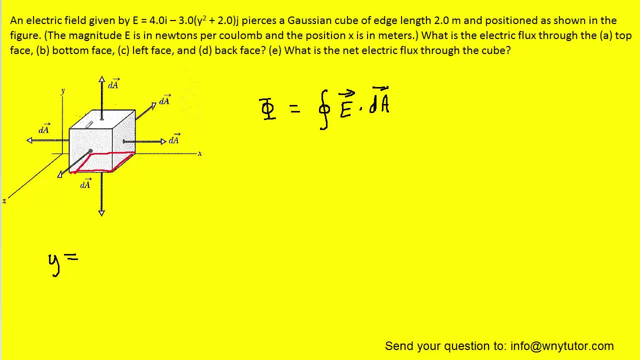 but in order for there to be an electric flux to the back face of the cube, we're going to have to be an electric field component that's streaming through the back face. in other words, there would have to be an electric field component along the z axis and that way electric field lines would 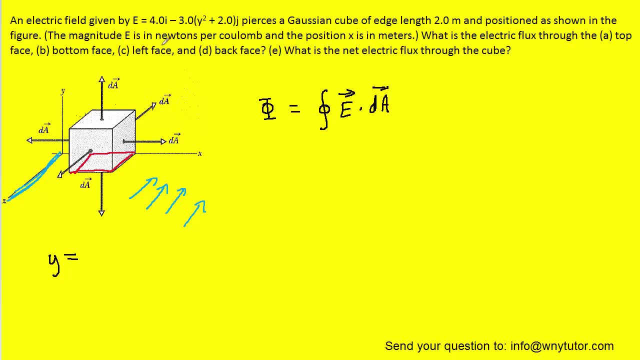 actually be flowing through the back face. but we can see from the electric field equation that, because there's only i hat and j hat, that there is no electric field component in the z direction and if there's no electric field in the z direction, there's no electric flux flowing through the back.